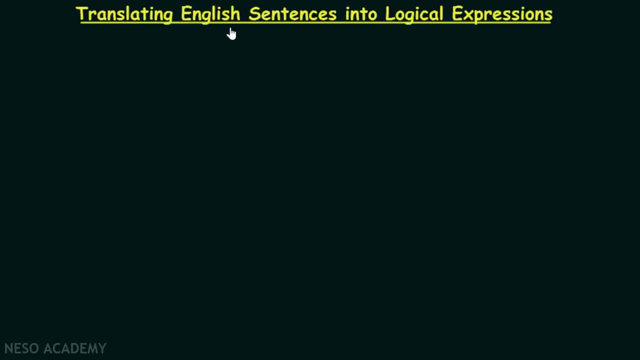 In this lecture, we will learn how to translate English sentences into logical expressions. Now, why do we need to convert English sentences to logical expressions? There are, of course, multiple reasons to translate English sentences to logical expressions. Let's consider few of them. 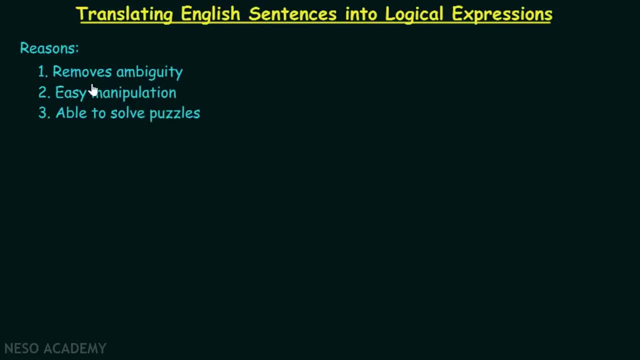 First of all, it removes ambiguity. This is the major reason why we are translating English sentences to logical expressions. It is possible in a language like English, where a particular sentence has multiple meanings. In mathematics, this is not something which is acceptable. Therefore, removing ambiguity, 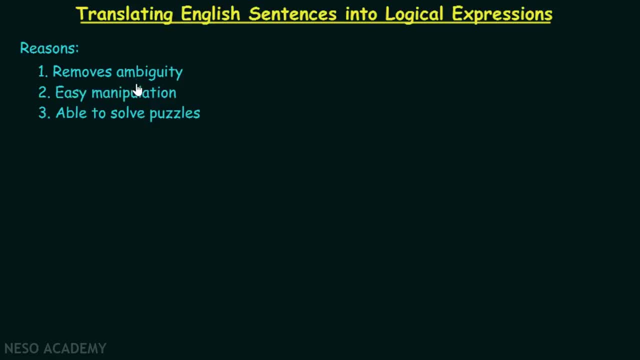 is very important and hence we convert English sentences to logical expressions. Now, the second most important reason is that it is quite easy to manipulate logical expressions in comparison with English sentences. English sentences are not easy to manipulate with, On the other hand, logical expressions. 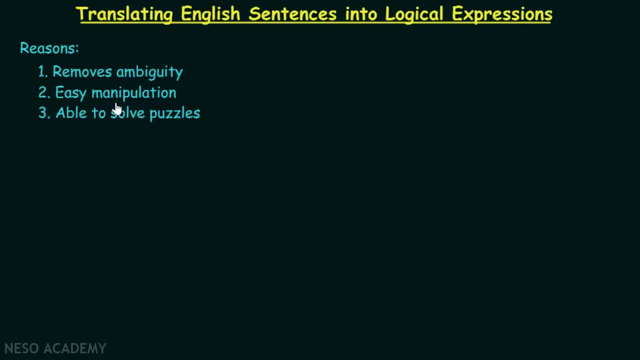 are quite easy to play with. We would be able to reason about sentences or mathematical statements very easily using logical expressions in comparison with English sentences. And the third reason is we would be able to solve puzzles very easily if we consider logical expressions instead of English sentences. 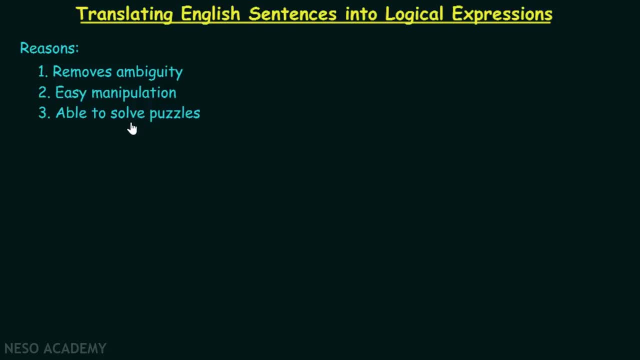 Now let's consider one example in order to understand. how do we able to convert English sentences to logical expressions? You are not allowed to watch adult movies if your age is less than 18 years or you have no age proof. Now the first step. 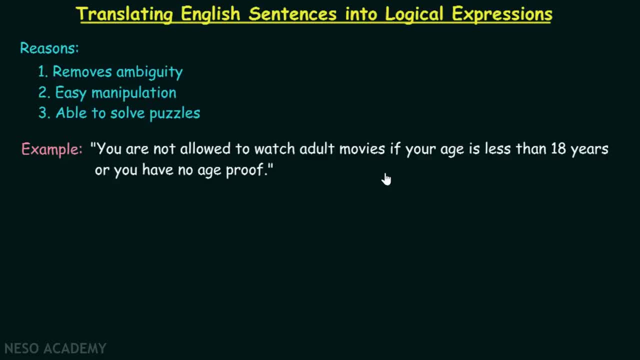 that we need to follow in order to convert this English sentence into a logical expression is as follows: Find the connectives which are connecting the two prepositions together. In order to convert this English sentence, we first need to find out the connectives which are joining the two prepositions. 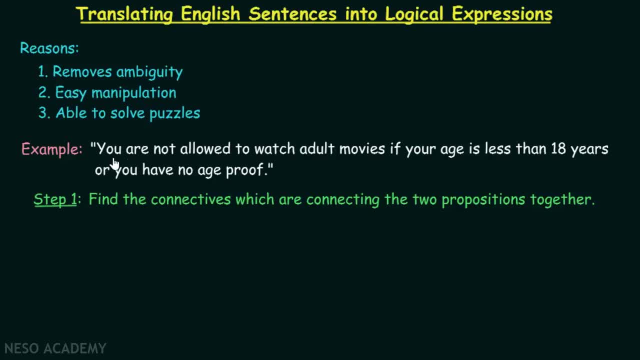 together. Like we can easily see that this is one preposition. You are not allowed to watch adult movies, And this is the compound preposition- your age is less than 18 years or you have no age proof. These two prepositions are connected. 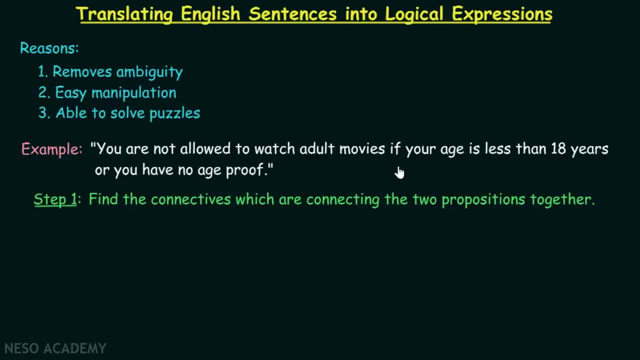 together using, if, construct. Isn't that so? So this is one connective. Now, this compound preposition is connected by using, or Right Now. the second step is to rename the prepositions In this sentence. not only we find out the connectives, 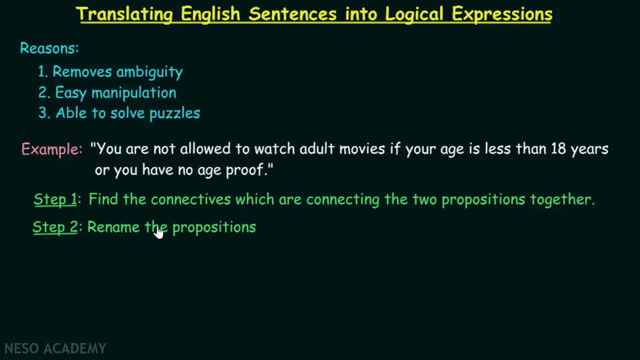 but also the prepositions. Now our job is to rename these prepositions one by one. Let Q is you are allowed to watch adult movies. R is your age is less than 18 years. S is you have age proof. Now we are all set to convert. 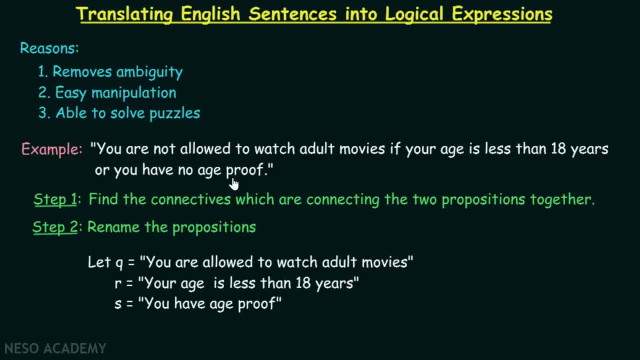 this English sentence into a logical expression Here, as we know that this particular statement is of the form Q. if P Isn't that so, Which is equivalent to if P, then Q That means P implies Q. If suppose this whole compound preposition is P. 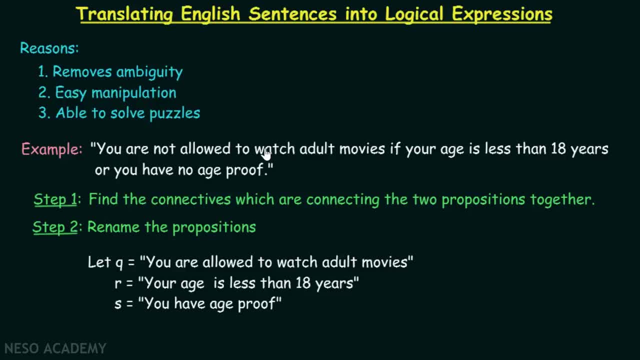 then this statement is of the form P, implies, not Q, Because here, as we can see, Q is you are allowed to watch adult movies, But here it is written: you are not allowed to watch adult movies. Therefore, this statement is of the form P, implies not Q, Right? 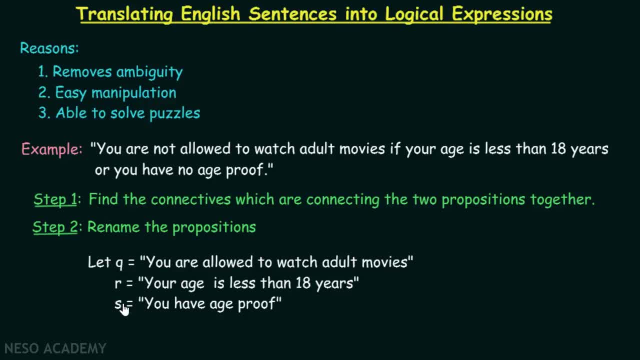 So what is P? P is R or not S, Isn't that so? As R is the preposition your age is less than 18 years and S is the preposition you have age proof. So this statement: your age is less than. 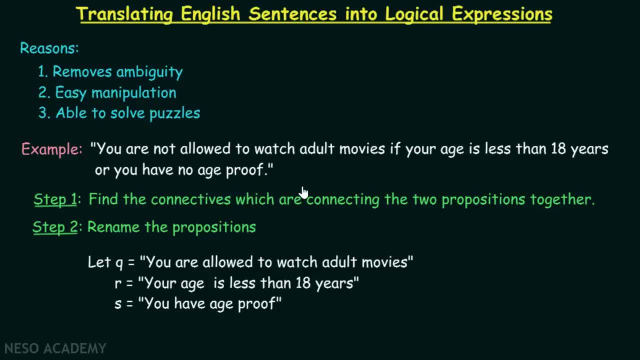 18 years or you have no age. proof is R or not S, Isn't that so? Therefore, logical expression for this English sentence would be: R or not. S implies not Q. Now let's consider one problem: Are these system specifications consistent? 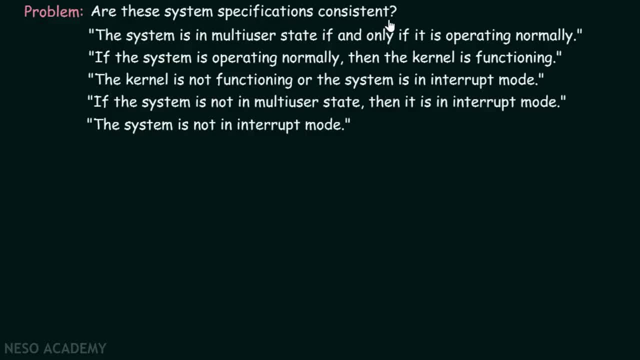 We will understand the meaning of consistent later on, But let's first consider all the system specifications. The system is in multi-user state if, and only if, it is operating normally. If the system is operating normally, then the kernel is functioning. The kernel is not functioning. 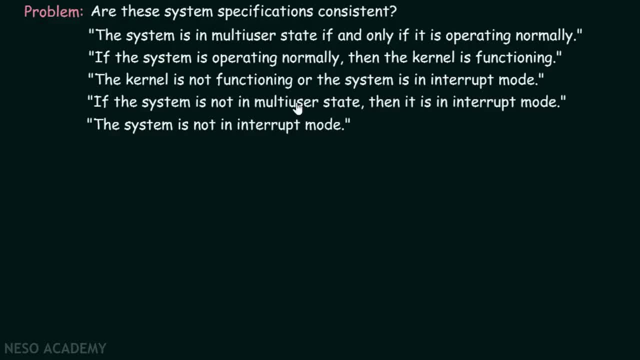 or the system is in interrupt mode. If the system is not in multi-user state, then it is in interrupt mode. The system is not in interrupt mode. These are all the system specifications. Our job is to find out whether these system specifications are consistent or not. 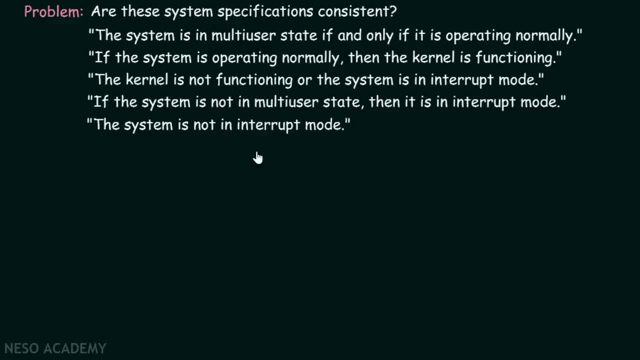 In order to find out whether these system specifications are consistent or not, our first job is to convert these specifications into logical expressions. We already learned that. how do we able to convert these English sentences to logical expressions? Let's say: P is. the system is in. 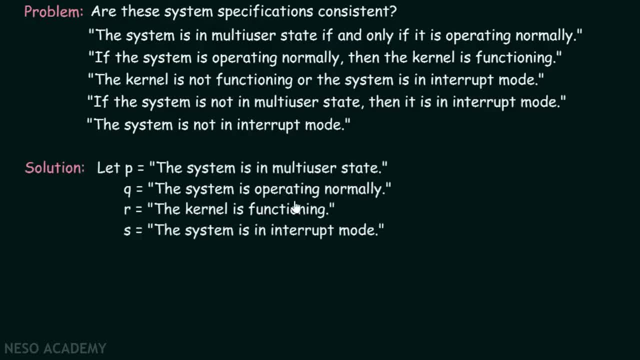 multi-user state. Let Q is the system is operating normally, Let R is the kernel is functioning and S is the system is in interrupt mode. Let's start from the first statement itself and try to convert this statement to a logical expression. The system is in multi-user state. 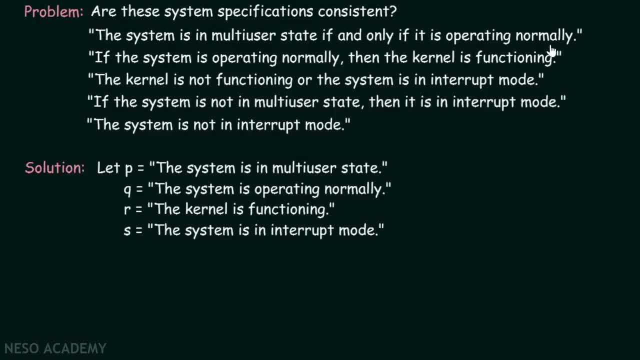 if, and only if, it is operating normally. Now, how do we convert it into a logical expression Here? as we know, P is the system is in multi-user state and Q is the system is operating normally. Therefore, this statement is of the form. 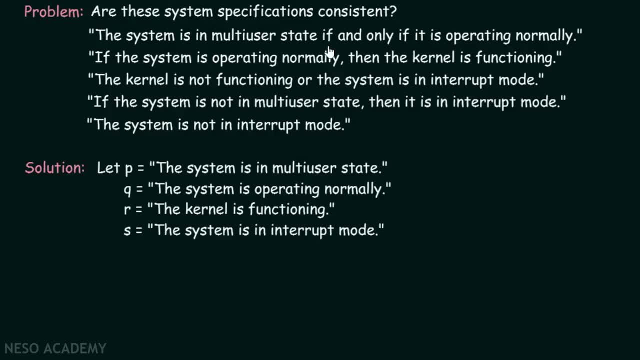 P, if, and only if, Q, And hence the logical expression corresponding to this particular sentence would be P. bi-conditional operator: Q. Right, We need to put bi-conditional operator to indicate if, and only if. Okay, now let's consider the next sentence. 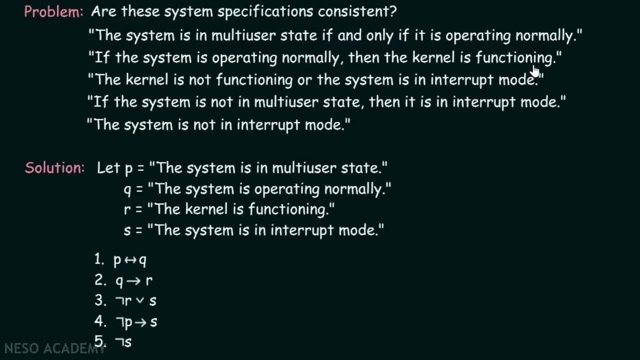 If the system is operating normally, then the kernel is functioning. As Q is the system is operating normally and R is the kernel is functioning. Therefore, this statement is of the form: if Q, then R. Right, Which is equivalent to Q, implies R. 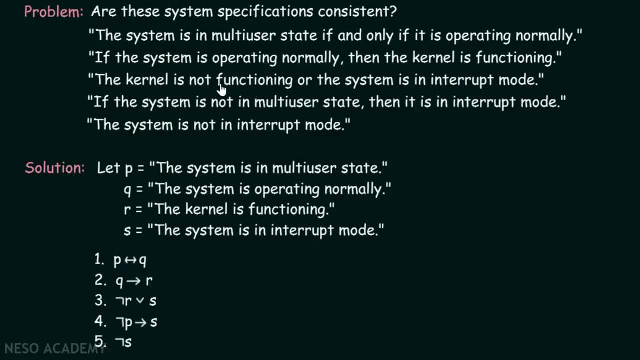 Let's consider the next sentence. The kernel is not functioning or the system is in interrupt mode. As R is, the kernel is functioning. Here we are saying: the kernel is not functioning. So this is not R, Or the system is in interrupt mode. 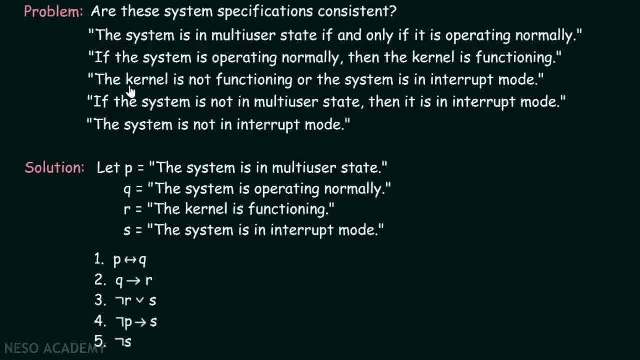 which is equivalent to S. Therefore, this statement is of the form, not R or S, Right? Similarly, you would be able to observe that this statement is of the form, not P implies S and this statement is not S. Okay, Now let's try to understand. 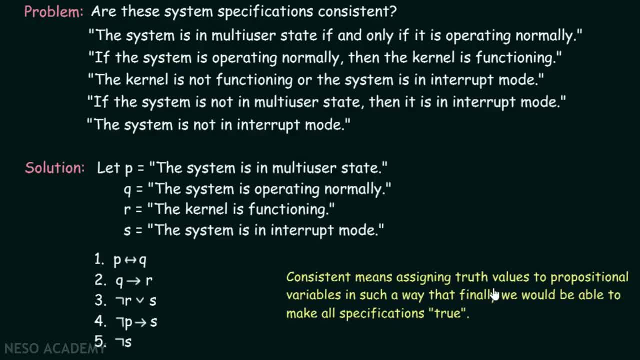 what is the meaning of consistent? Consistent means assigning truth values to propositional variables in such a way that, finally, we would be able to make all specifications true. This is the meaning of consistent. Consistent simply means that we need to make all these specifications true. 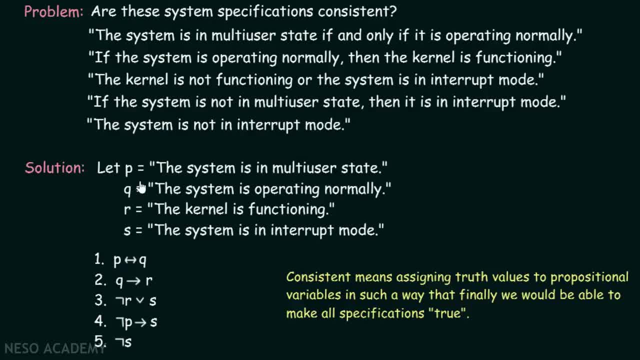 by assigning some truth values to propositional variables P, Q R and S. Whatever the truth values of P Q R S we choose, our ultimate job is to make all these specifications true. This is what consistent means Right. 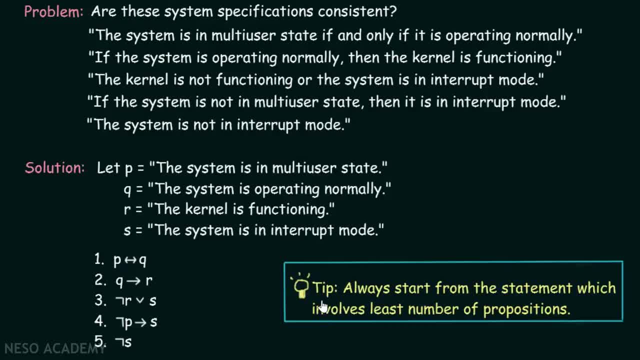 Now, how do we start? There is one tip that I would like to give you: Always start from the statement which involves least number of propositions From these logical expressions, not S involves the least number of propositions. Therefore, it is better to start from: 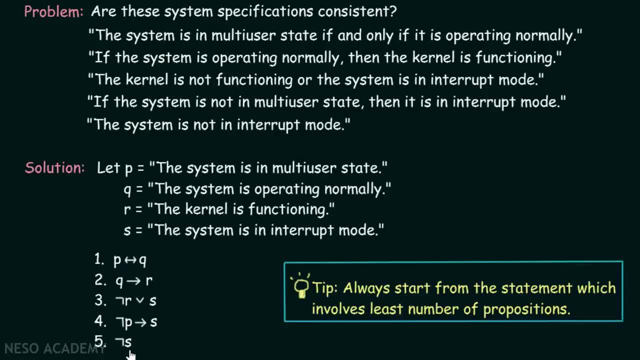 this particular proposition. Try to make this proposition true and then move to other statements. Okay, Now let's try to make not S true. Not S can be true when S is false, Isn't that? so When S is false, then only not S can be true. 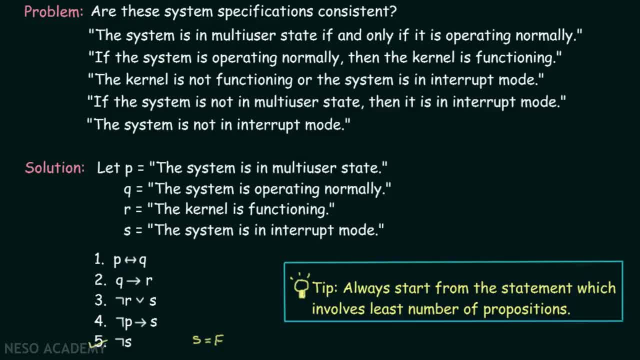 Therefore, we are successful in making this proposition true. Right, As S is false, then not P has to be false in order to make this compound proposition true, Isn't that? so Now, to make not P false, P has to be true. 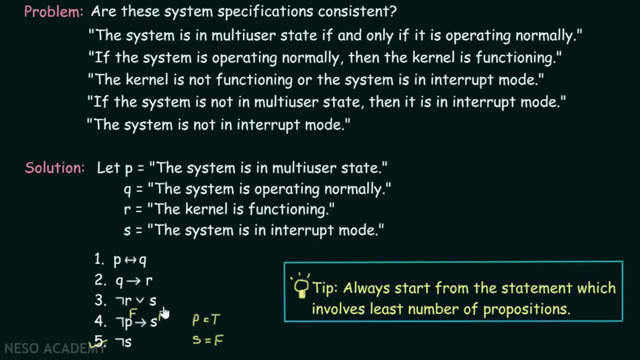 Right. Okay, Now we know that S is false. Right As this is false, this has to be true in order to make this proposition true. Therefore, if not R is true, then R would be false Right Now, as R is false. 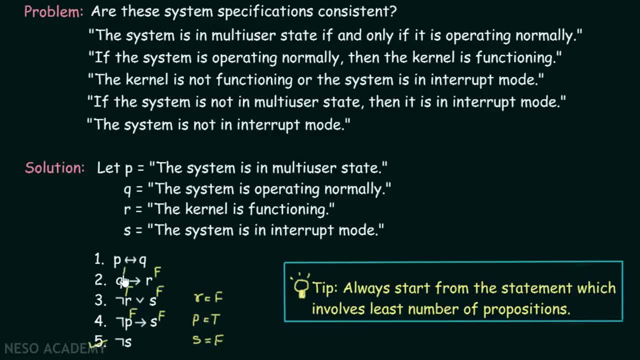 if this is false, this has to be false. Therefore, Q is also false, And we know that P is true and Q is false. We would be able to make this proposition true, this one true, this one true, but we would not be able to make.